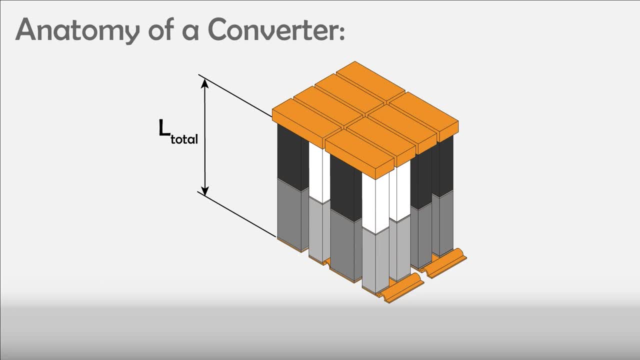 thermoelectric materials, the total unicouple height, the height of the high-temperature n-type material, the height of the high-temperature p-type material, the area of the n-type material, the area of the p-type material and load resistance. NASA is currently evaluating new 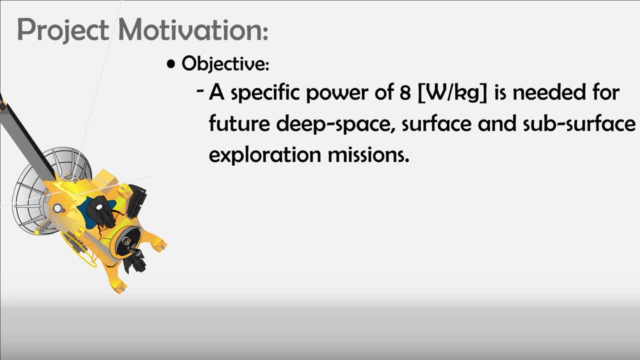 power sources and re-evaluating existing power sources. to be able to successfully complete new deep space and subsurface exploration, A specific power of 8 watts per kilogram is desired to complete most mission objectives. RTGs, although having flight-proven performance, currently have a specific power of about 5 watts. 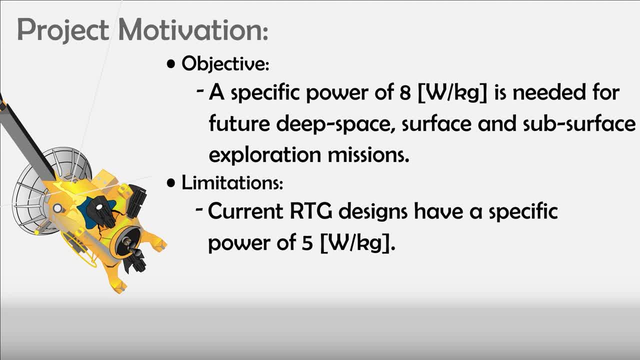 per kilogram. Thus, new heat sources and converter configurations need to be designed and evaluated. Given the large number of independent variables when designing and optimizing unicouples and current limited design methodologies, determining converter configurations that maximize specific heat sources and converter configurations are important, These unicouples 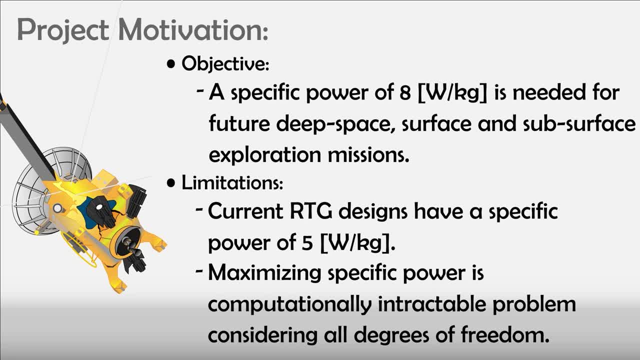 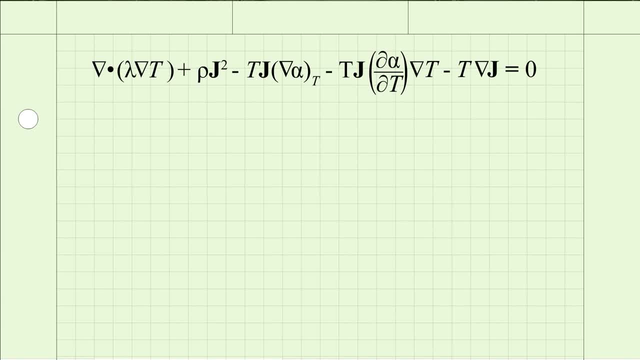 need to be designed and evaluated To optimize the thermoelectric converter geometry to maximize specific power. I first focused on the unicouple To model the temperature-dependent nonlinear thermoelectric effects occurring within the thermoelectric materials. I derived a novel analytic model from first principles. 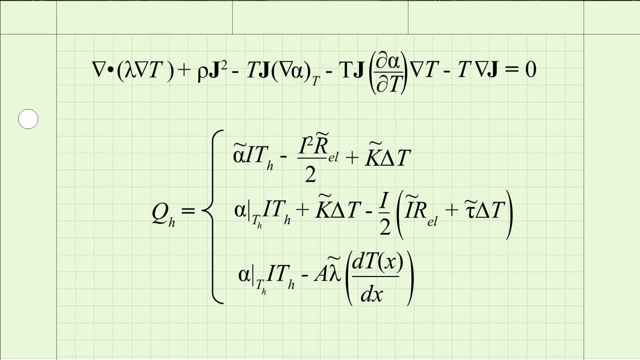 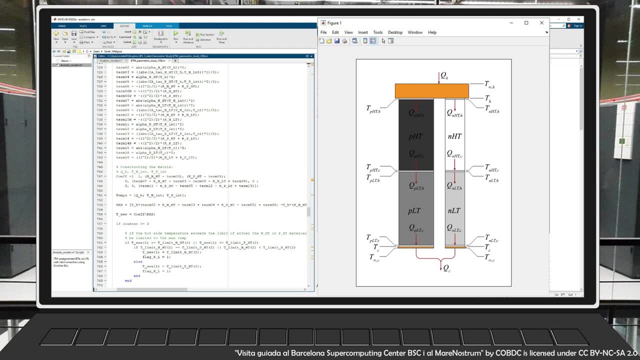 and evaluated two other existing analytic models. These models quantified the simultaneous thermal and electrical behavior of a segmented unicouple. I then coupled these constitutive equations to a thermal resistance network describing the unicouple. The thermal resistance network allowed for consideration of the thermoelectrical resistances. 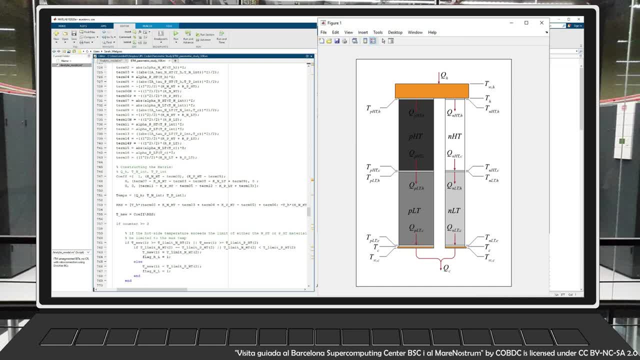 of interconnectors, the joule heat generated within the interconnectors and contact resistances between the materials. By doing such, I created a thermoelectric-coupled iterative mathematical model that was then implemented in MATLAB. This model could handle Dirichlet in mixed 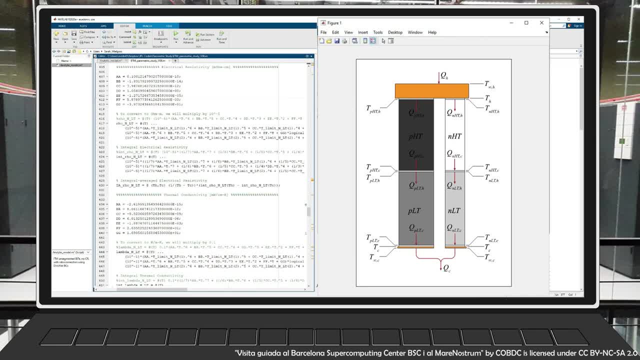 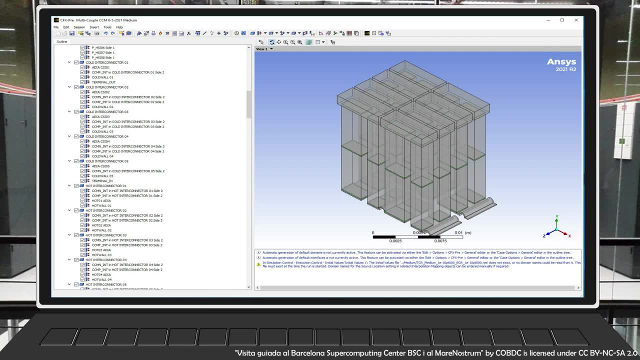 thermal boundary conditions to simulate converter operation. The solve time of this model was on the order of tens of milliseconds on a single core. To validate my analytic models, I developed a high-fidelity three-dimensional fully-coupled finite-volume model in ANSYS-CFX. Using cell expressions, I was able to couple all thermoelectric 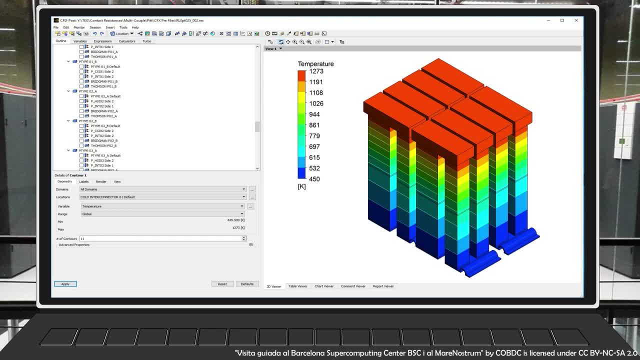 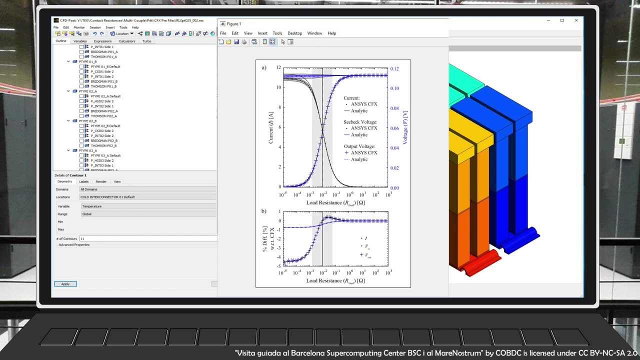 effects to the energy equation, considering temperature-dependent material properties, and allow for the implicit evolution of electric boundary conditions. with the solution, The latter decreased solve time, which was on the order of minutes. using a three-dimensional, 32-core node, Agreement between the numeric and analytic models was within 1%. 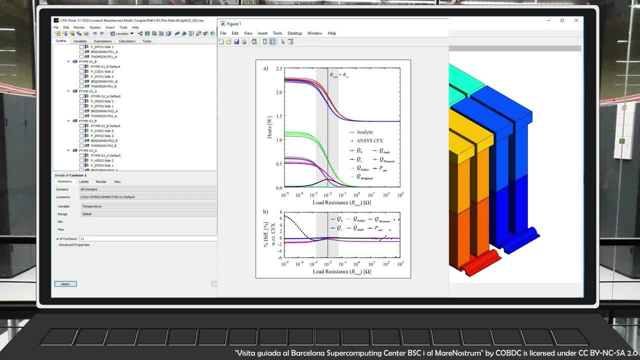 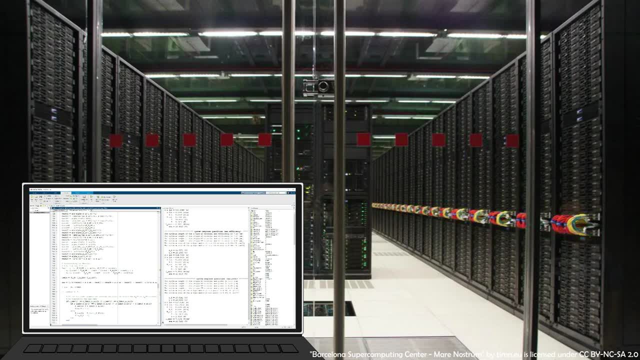 Once I established confidence in my models, I undertook evaluating the entire design space- over 100 billion unique converter configurations. I conducted a full parametric study considering the 10 independent variables and over 100 billion converter configurations, to find the maximum achievable specific power and to benchmark my fast-compute algorithms against. 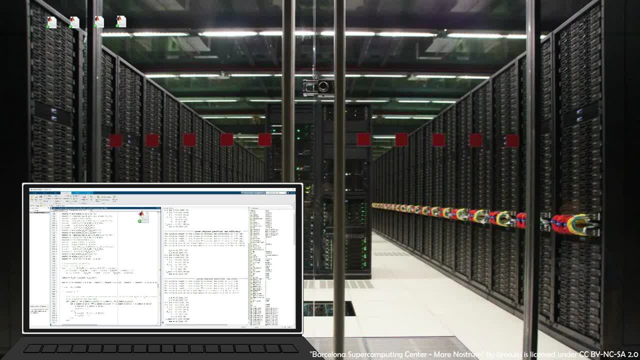 To complete this task, I used a number of parameters to find the maximum achievable specific power and to benchmark my fast-compute algorithms against. To complete this task, I used a number of parameters and to benchmark my fast-compute algorithms against. To complete this task, I used a number of parameters to find the 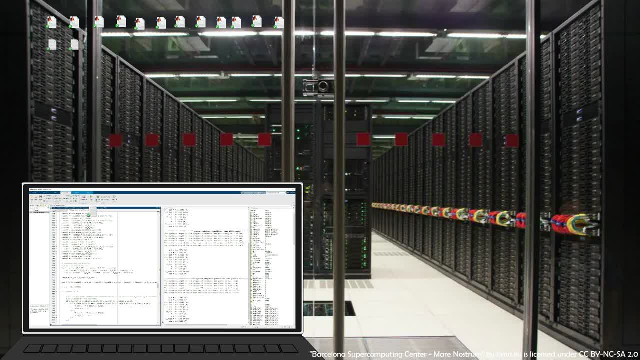 maximum achievable specific power and to benchmark my fast-compute algorithms against The processes should require the strongest collections of complex чисじゃあ in thehwa inch. I used MATLAB to automatically break down the design space and generate numerous unique functional input versions of my code, known as Emfiles. 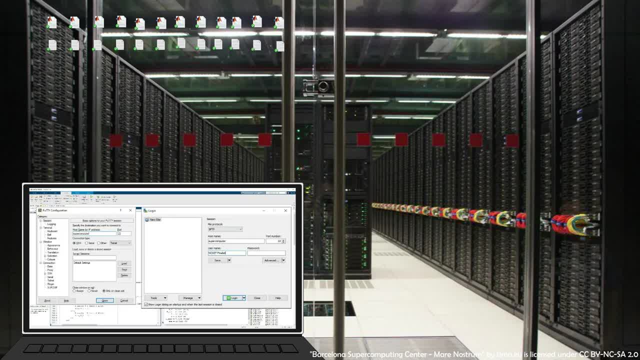 I then use MATLAB to automatically generate unique Slurm files for each distinct EMS file, such that the MATLAB code could be run on the supercomputer's Linux operating system, Using MATLAB's programming environment to manage thousands of versions of my code on the supercomputer via WinSCP and PuTTY, I was able to run 5,000 instances of the code. 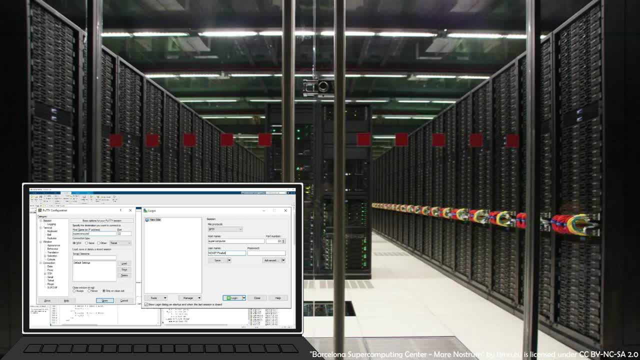 minimal user input. The average solve time of each individual mfile, each of which was considering over 10 million converter configurations, was on the order of days Without the fast, compute analytic models I developed previously and without decomposing the design space to thousands. 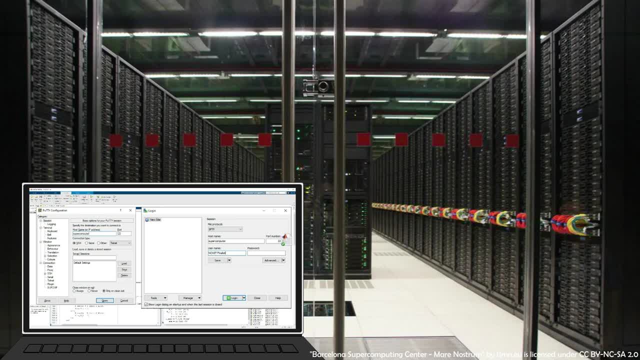 of subspaces. solving this problem would have been impossible. Once the codes finished running, I collected and analyzed the results. Using MATLAB, I parsed the results and found the optimum configuration that maximized specific power. But this wasn't the best approach, Not. 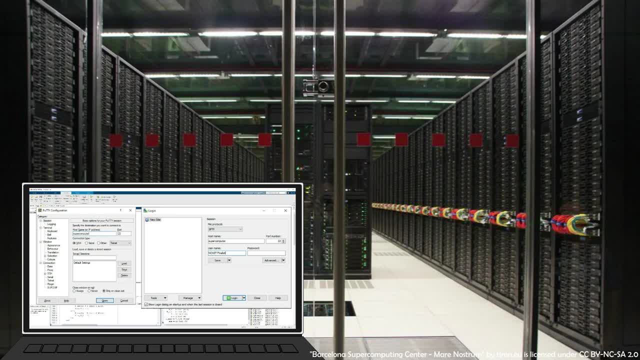 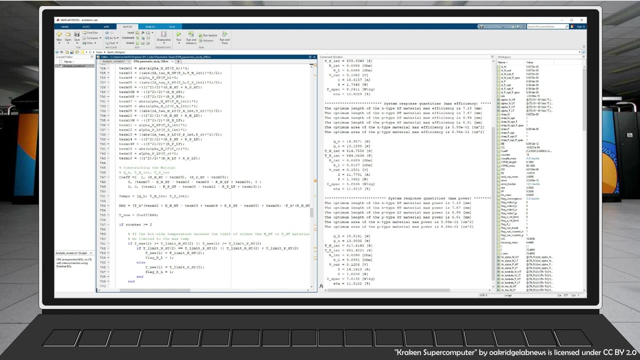 everyone has access to a supercomputer. I wanted to make the code run faster with fewer computational resources needed, all the while without sacrificing fidelity. I had to develop fast compute algorithms. I implemented a variety of algorithms to reduce runtime, to make the code more accessible. 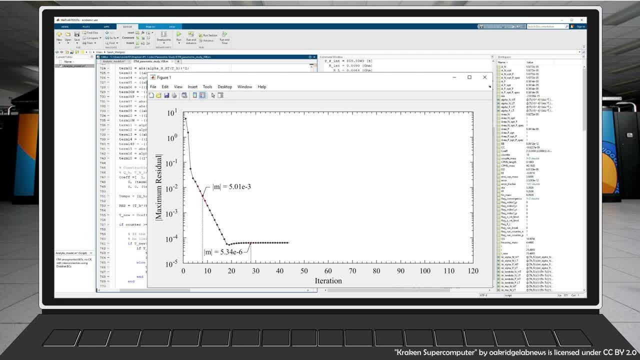 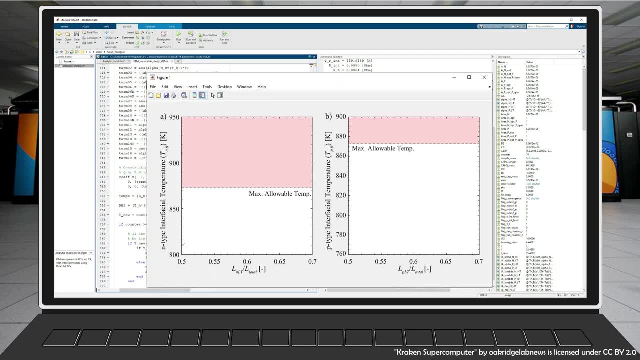 The first was a residual tracker Through use of a central differencing scheme. the code would terminate if the residuals failed. Next, I implemented a machine learning algorithm that limited and redefined the design space range, based on previous solutions that violated design constraints such as maximum segment.